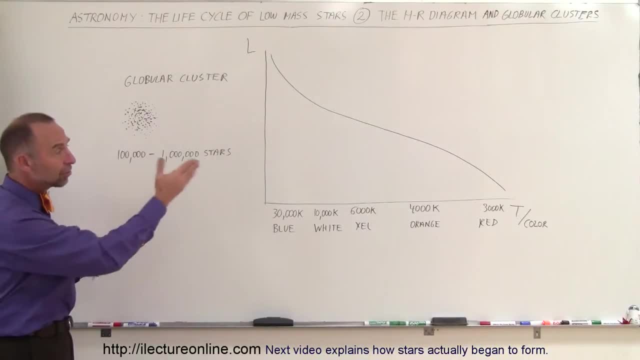 did was we looked at the color, the temperature of the star and then placed it on the HR diagram And, based upon doing that, we saw something very, very interesting. Now, what's unique about these globular clusters is that pretty well all the stars in the globular cluster 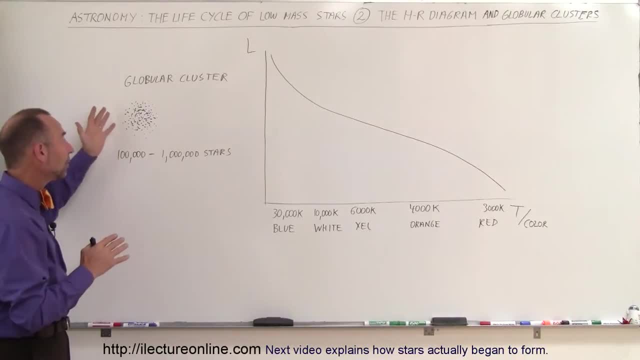 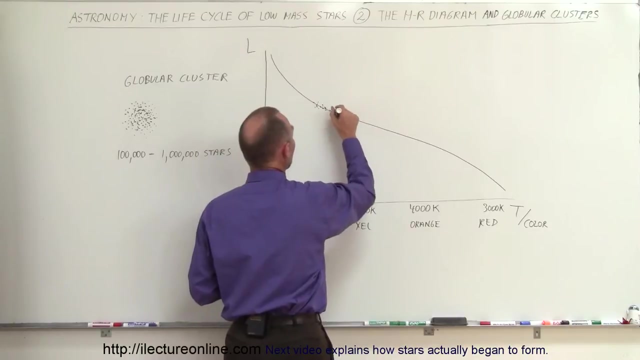 formed at about the same time, So they all were born around the same time from the same huge cloud of dust and gas. So we went to the H-R diagram and we saw something as follows: We found that a great number of them were still situated on the H-R diagram. 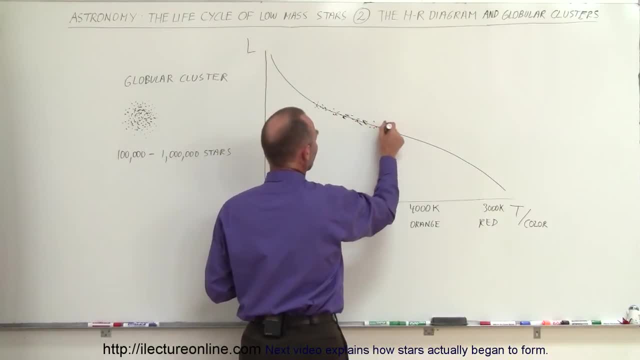 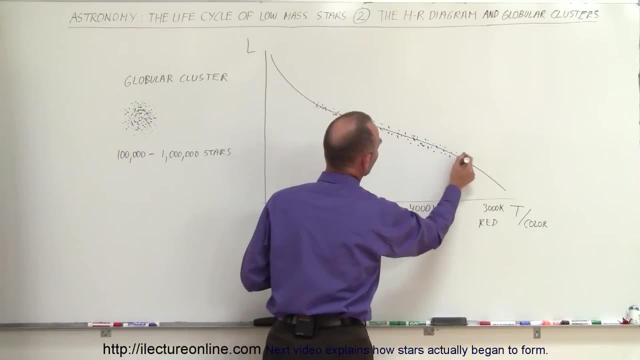 Well, this is going to take a little while, but let me try to illustrate So many. many of these stars were still clustered on the main sequence, And so what that meant was that they were still fusing hydrogen into helium in their cores. 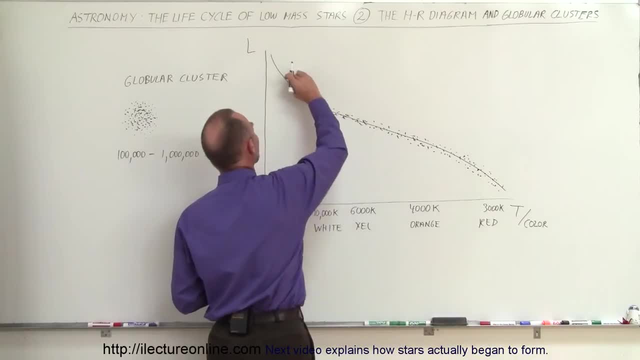 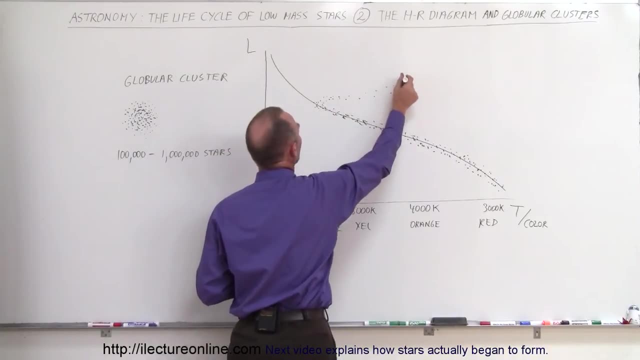 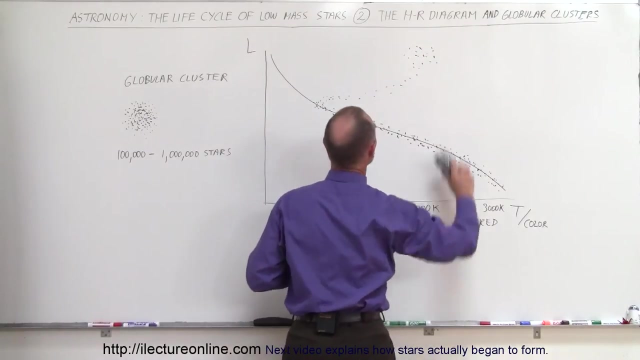 But what happened was there was a point where all of a sudden there were no stars past that point on the main sequence, but the stars seemed to veer off in the main sequence and end up something like this: A whole bunch of stars like that, And I guess I should actually 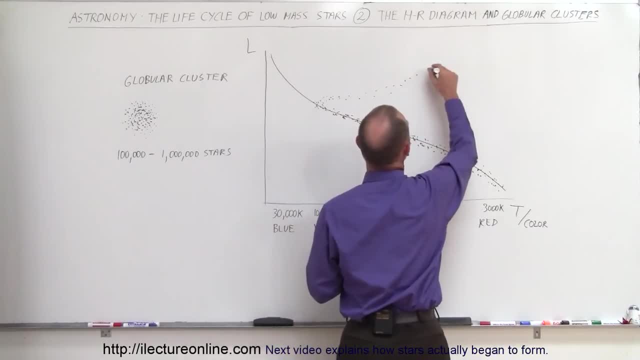 move it over just a little bit more. Let me go a little bit more over here, Alright, that would be a better position for them. And we had maybe some stars over there, And then we had some stars that were located over here. 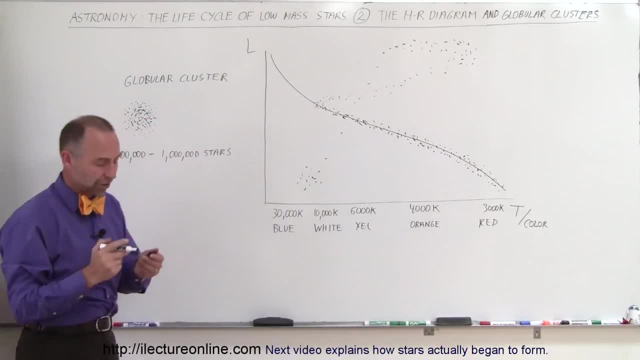 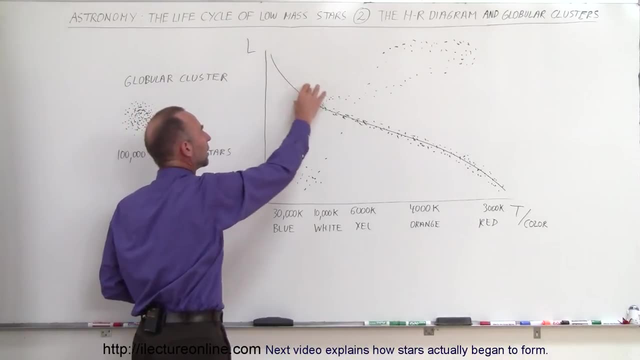 Now that's the H-R diagram. That's pretty well what we normally would see on an H-R diagram, except on a regular H-R diagram when we looked at stars from all over, we'd also see a bunch of stars over here. Notice that they were completely devoid, And this point here is known as the turn-off. 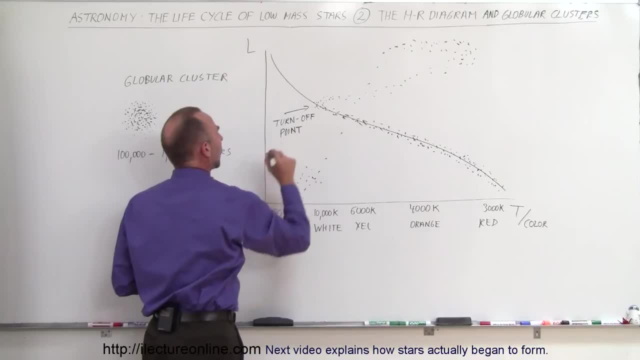 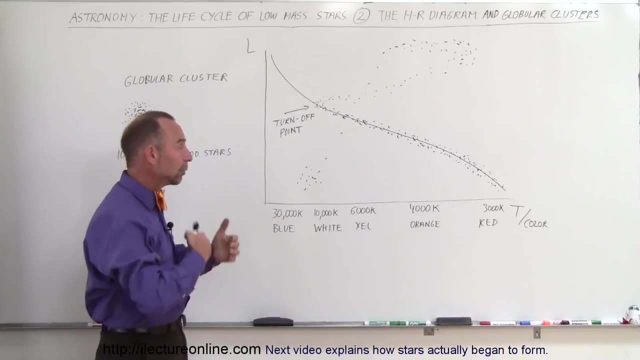 point Now. what we also discovered was that very large stars that are on the main sequence, the big blue stars, with very high temperatures. they would burn through their nuclear fuel very, very fast. The core of these stars would be so hot that the nuclear fusion process where hydrogen was converted into helium, would go so fast that they would only spend a fairly short amount of time as a main sequence star, Maybe as much as 50 or 100 million years, And then they would go through their red giant stage. 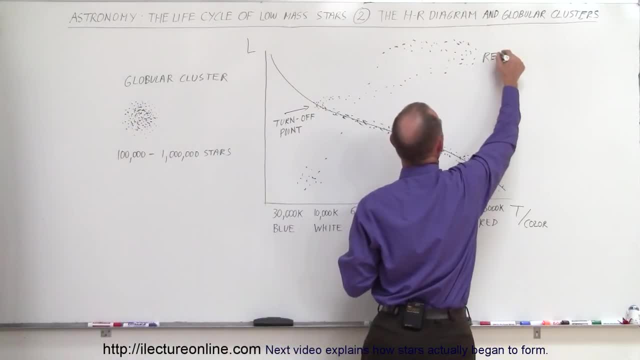 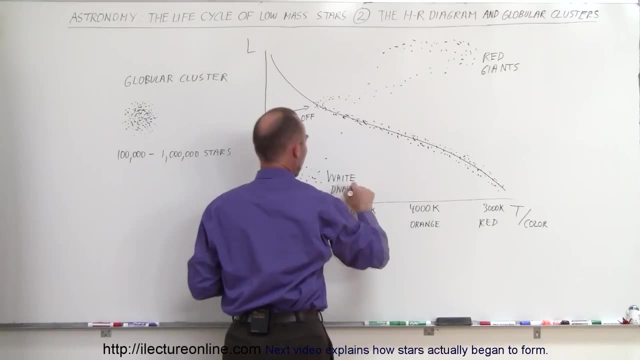 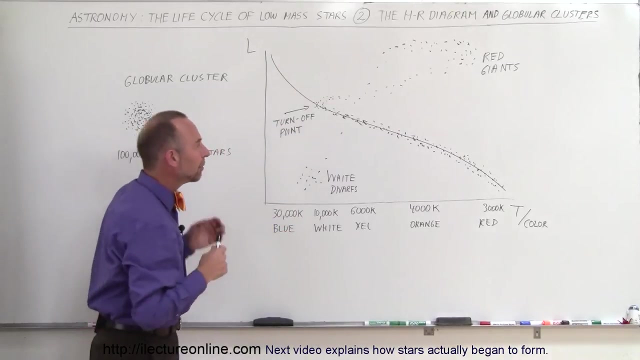 So the stars over here were known as red giants, The stars down here in the left corner were known as white dwarfs, And so what we could do with the turn-off point is we could realize how long a star could survive on the main sequence as a main sequence star before. 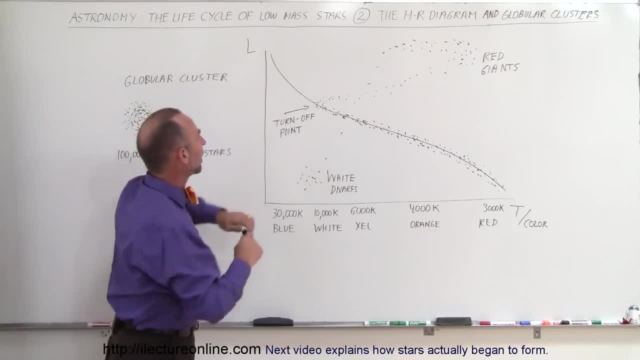 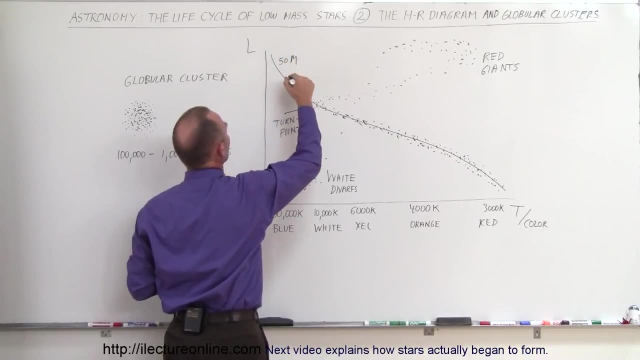 it would turn itself into a red giant And we would say that any stars that are up here, they would only last maybe about 50 million years, So maybe I'll write as 50 with an M. And stars over here maybe 500 million years, And over here 1 billion year And here 3. 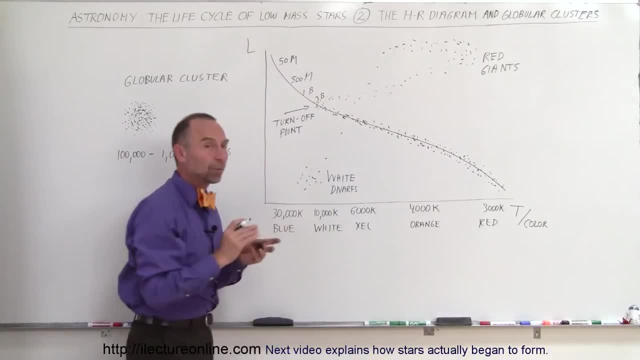 billion years. So what that means was, if the turn-off point was at a position where stars would no longer remain on the main sequence, they would then finish their main sequence stage after 3 billion years And then they would go through their red giant stage And 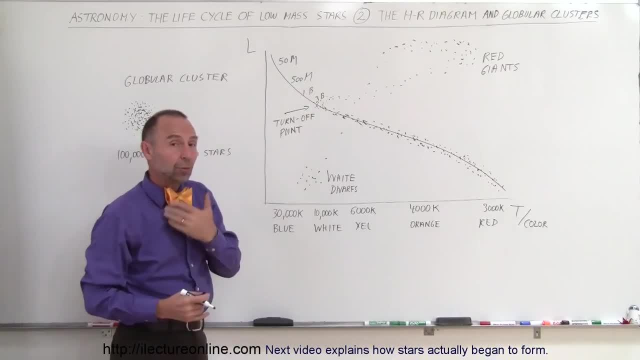 this was a really good example of a cross-referential approach. So, any stars that were less than 3 billion years old, that would tell us that this star cluster was about 3 billion years old, Because any stars that were older than 3 billion years old, Well, no, I'll take. 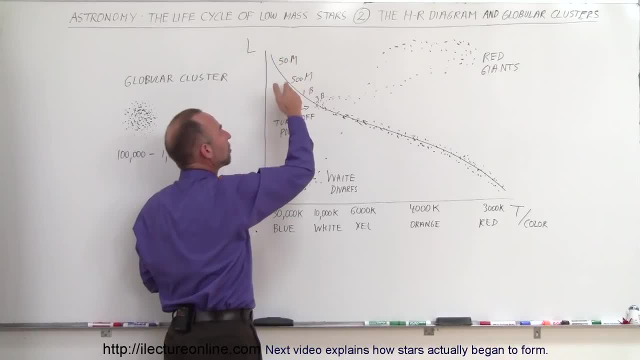 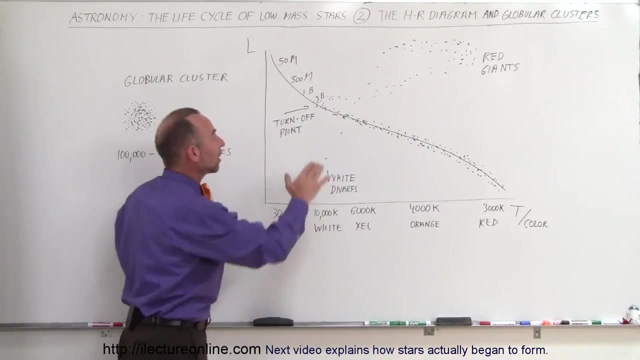 that back. Any stars that were less than 3 billion years old would have already changed from a main-sequence star into a red giant, And any stars that are smaller than that critical mass they need to go to a red giant stage. at this point in time they would still need. 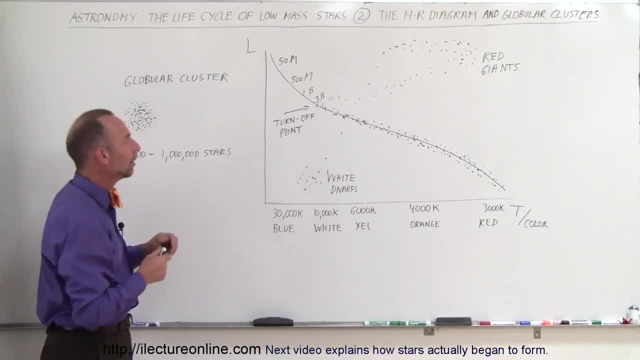 a few more billion years before they would turn into red giants, an indicator of how old the stars are in one of those clusters. and so, by looking at this, we began to see that the that the hr diagram, when you take all the stars from global cluster and put them on. 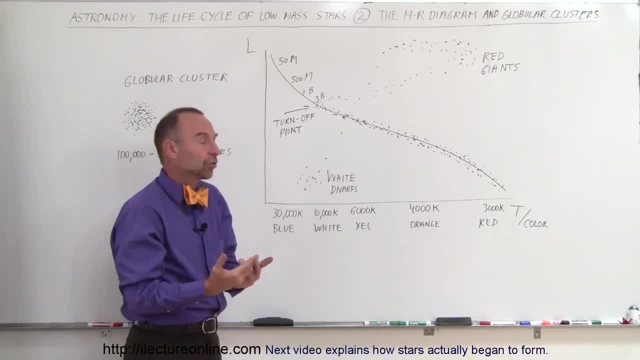 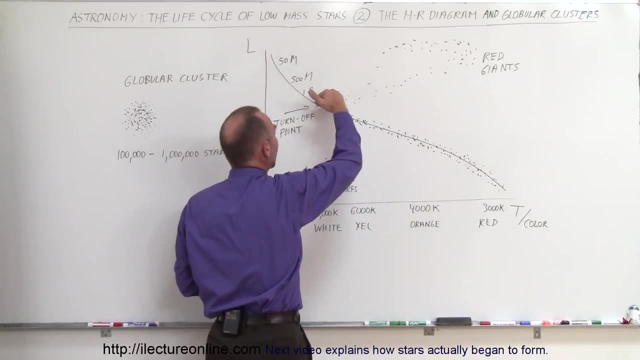 an hr diagram. it would tell- actually tell you- the life cycle of the star. you could see that stars would stay on the main sequence for a long time and after so many years, depending upon how big they were, they would then turn themselves into red giants, and then you could see that they would kind. 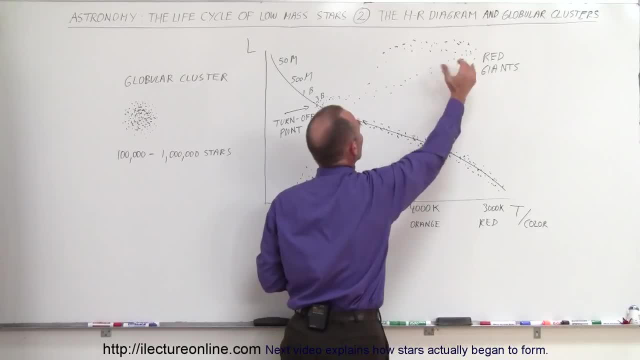 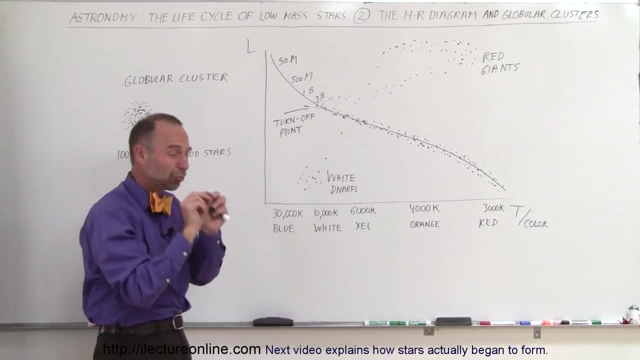 of change. there would be a period in which they reach the red giant stage, then there would be a stage in which they would change and then, finally, they would end up as white dwarfs. now, white dwarfs are very small, very dense, very hot stars surface is very hot, but they're very tiny. they have very 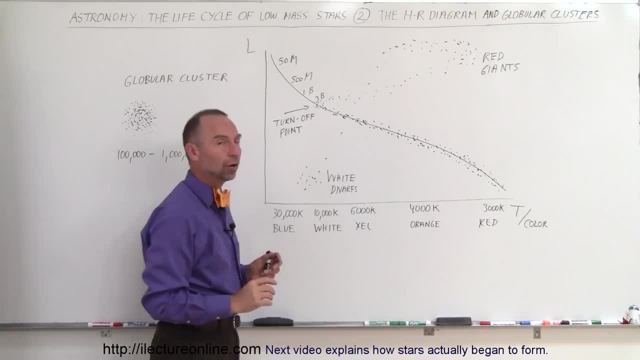 low luminosity, and that would then be the end stage of a star. so the hr diagram gave us a really good picture of the cycles of a star and how a star would change from one phase to another, and so what we're going to do in these videos is study the